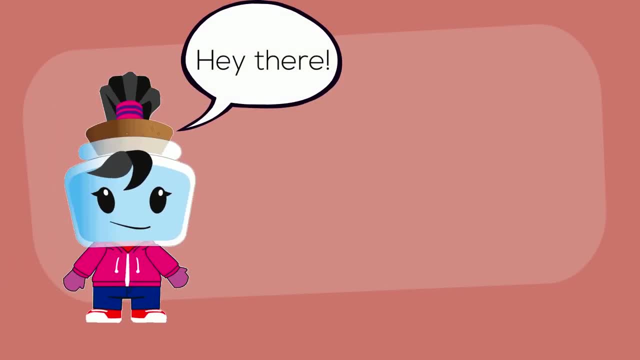 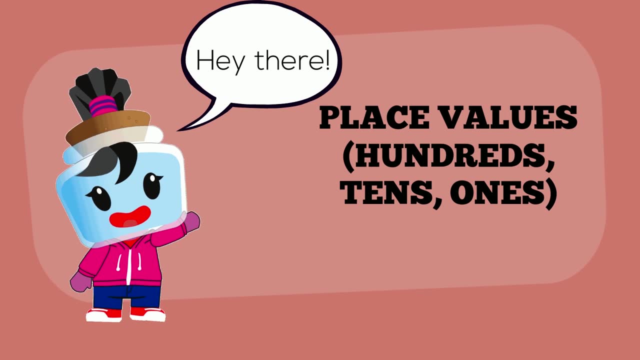 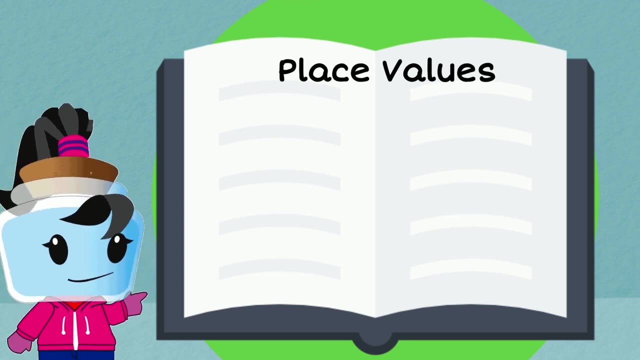 Hey there. Today we will be learning more about place values, In particular hundreds, tens and ones place values. Let's do a quick review of place values. Each digit in a number has a title depending on where it's positioned. In the number 43, we have four tens and three. 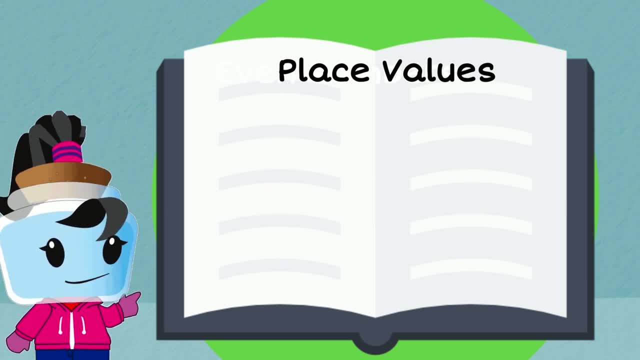 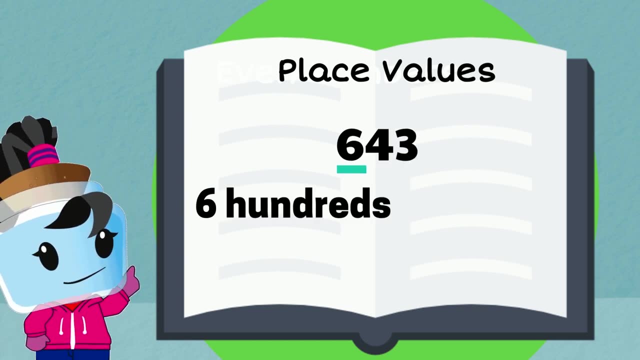 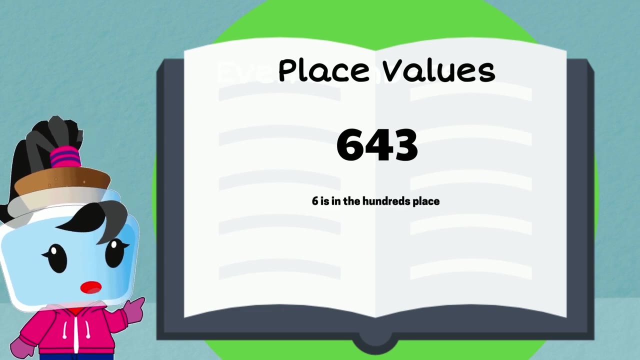 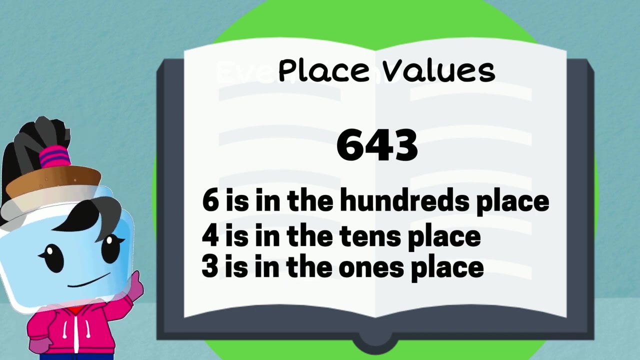 ones. Now, if we add another number and make it 643, we'll have six hundreds, four tens and three ones. In other words, six is in the hundreds place, four is in the tens place and three is in the ones place. Let's have a visual example by counting the blocks here. 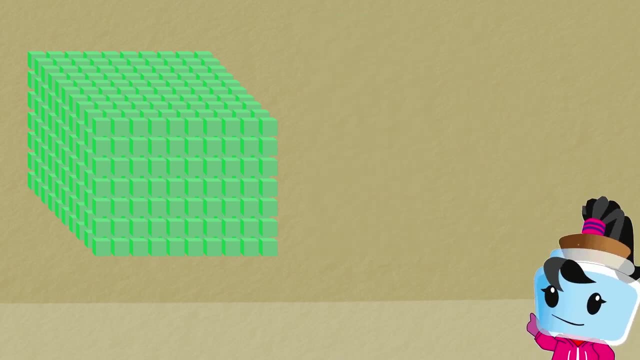 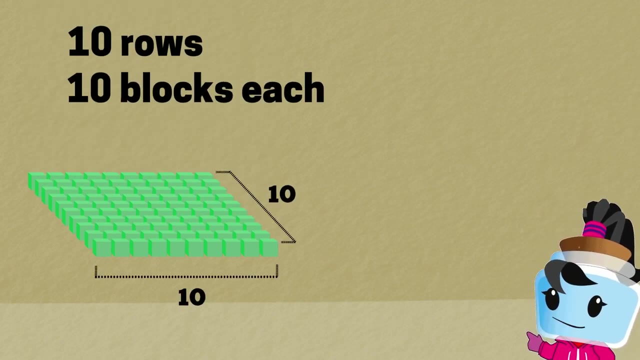 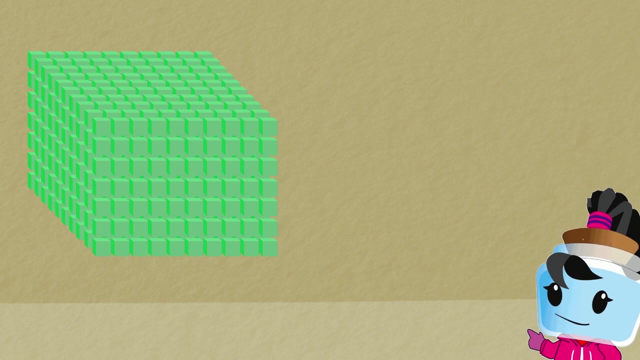 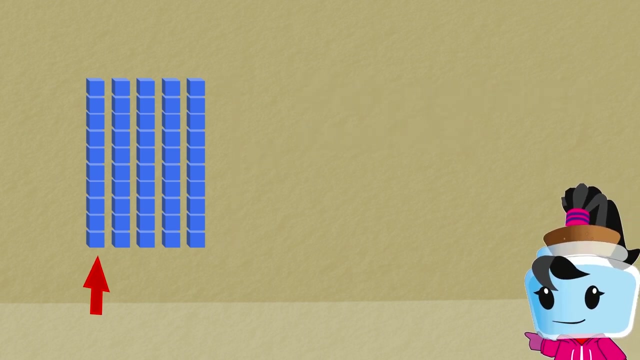 First notice the layers of the blocks. Since each layer has 10 rows of 10 blocks, we can say that each layer has 100 blocks. Next, let's look at the stacks of 10 blocks each. There are one, two, three, four, five stacks. 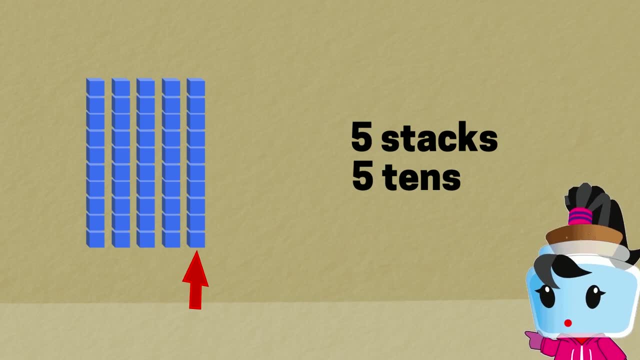 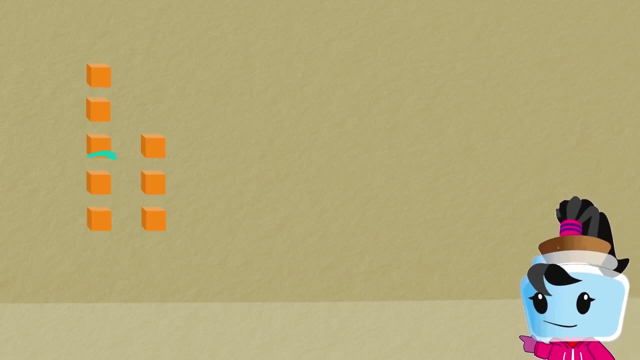 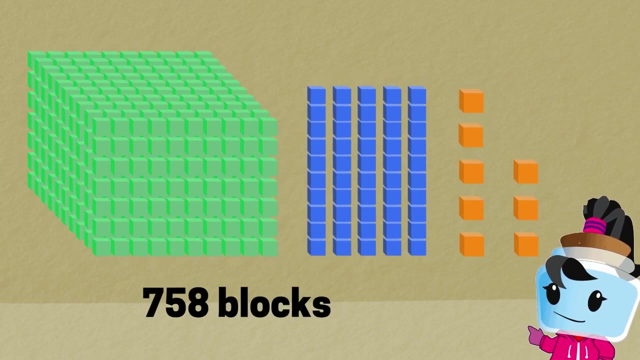 That means we have five tens. Lastly, let's count the separate blocks: One, two, three, four, five, six, seven, eight. So we have eight ones. Therefore, we have 758 blocks in total. Good job. 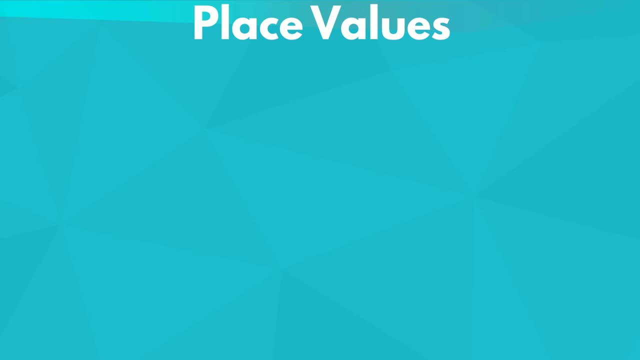 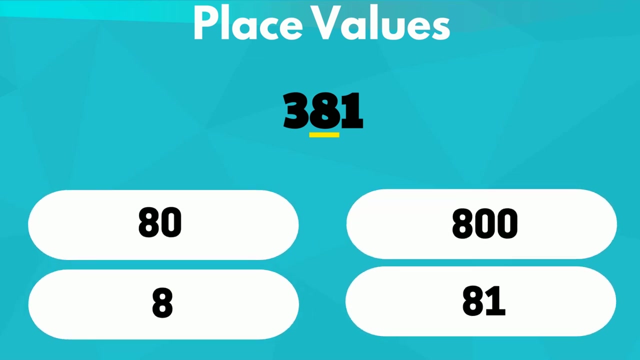 Let's do more practice on place values For the following numbers. choose the value of the underlined digit. The underlined digit eight is in the tens place, so its value is 80.. Next, Five is in the hundreds place, So its value is 500.. Next,